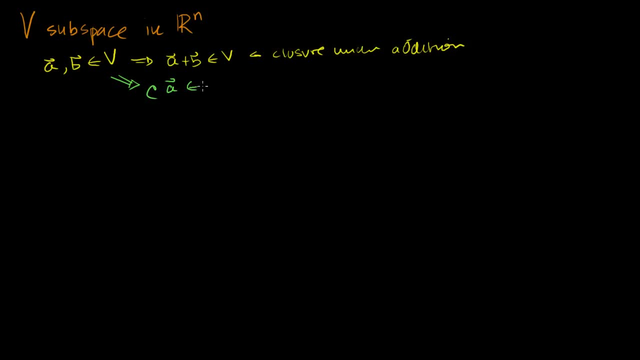 multiply A by some scalar, That this is also going to be a member of our subspace, And we sometimes call this closure under scalar multiplication. And then a somewhat redundant statement is that V must contain the 0 vector, And that's true of all subspaces. 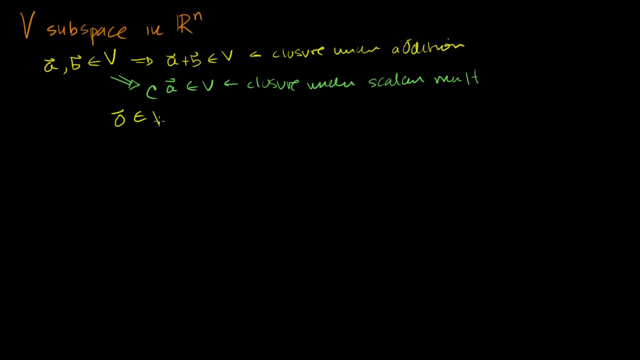 Let me write it this way: The 0 vector is a member of V And it would be the 0 vector with n components here. Because V is a subspace, It's a subspace of Rn. And why I say that's redundant? because if I say 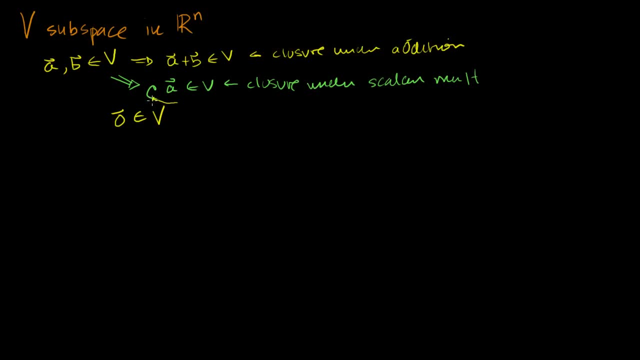 that any multiple of these vectors is also in V. I could just set the scalar to be equal to 0. So this statement kind of takes this statement into account. but in a lot of textbooks they'll always write: oh, and the 0 vector has to be a member of V. 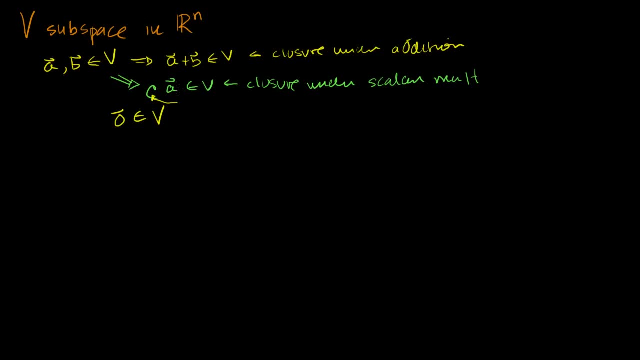 Although that's kind of redundant with the closure under scalar multiplication. Fair enough, Now let's say that I also have some transformation T. I have some transformation T. It is a mapping, a function from Rn to Rm. What I want to understand in this video is: I have a 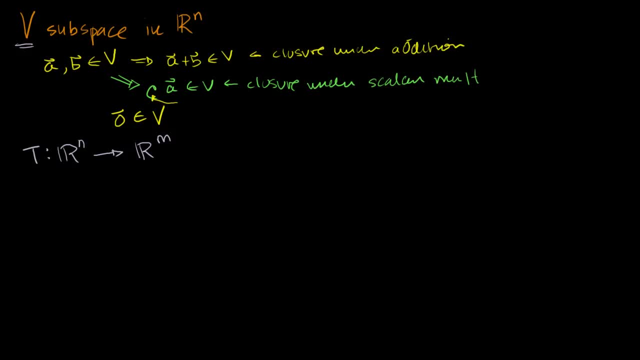 subspace right here V. I want to understand whether the transformation of the subspace so the transformation of the subspace, And what did we call that? We called that the image of our subspace Or our subset. either way, 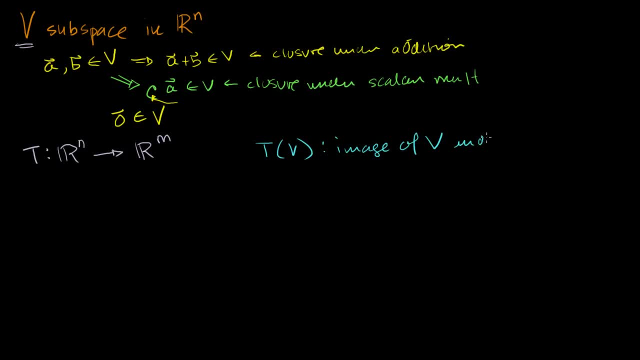 The image of V under T In the last video just to kind of help you visualize it. how did that work? We had some subset of Rn that looked like this. It was a triangle that looked something like that And that was in Rn. 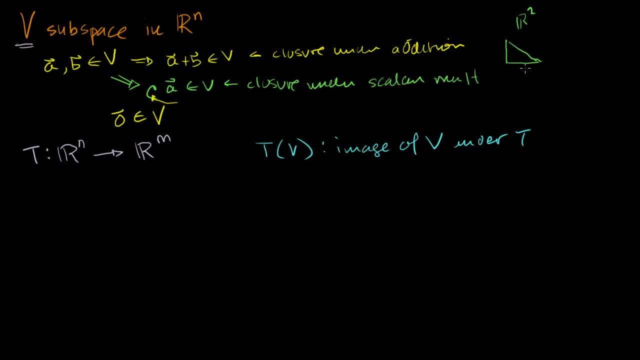 This was actually in R2.. It was a triangle that looked something like that And we figured out its image under T, So we went from R2 to R2.. And we had our transformation And it ended up looking something like this, if I. 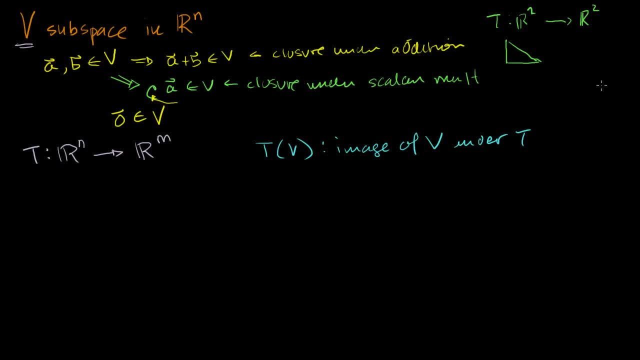 remember it properly, And it ended up looking like a. actually I don't remember it fully, but it was like a triangle that was skewed like this, rotated, So it was actually. I think it was more like. I think that's right. it was rotated a bit clockwise like that and it was. 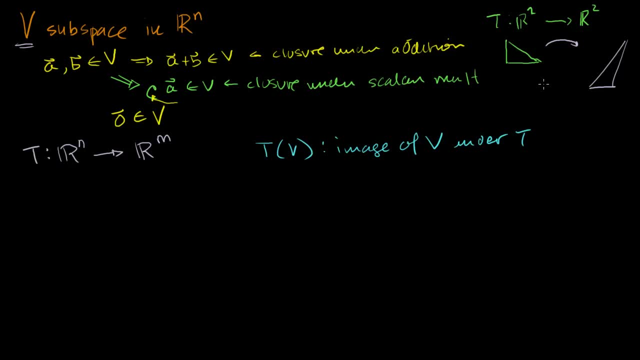 skewed. but the exact particulars of that last video aren't what matter. What matters is that you are able to visualize what an image under transformation means. It means you take some subset of R2, all of the vectors that define this triangle right here. that's some subset of R2.. 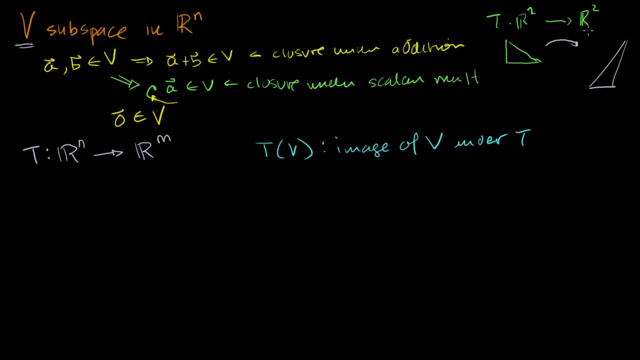 You transform all of them and then you get some subset in your co-domain And this is the. you could call this the image. you could call this the transformation of that triangle. Or if we call this s, it's equal to the transformation of. 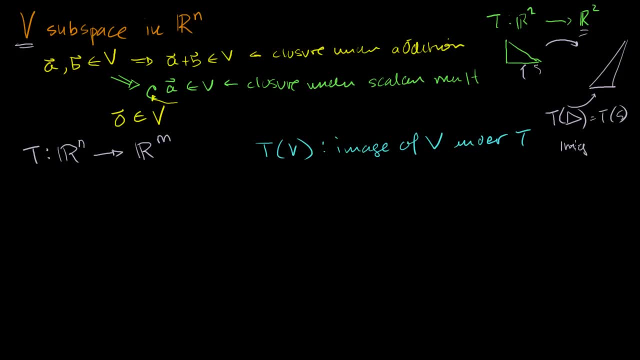 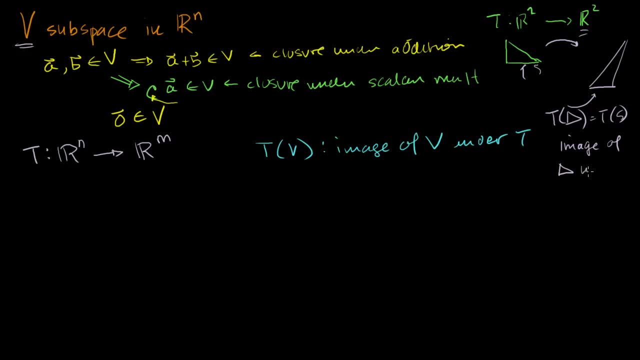 helps you to visualize. call it the image of this triangle under T, Or maybe even a neater way of thinking about it: is this triangle that skewed rotated triangle? this one is the image of this kind of right triangle under T And I think that might make a little bit of visual sense to 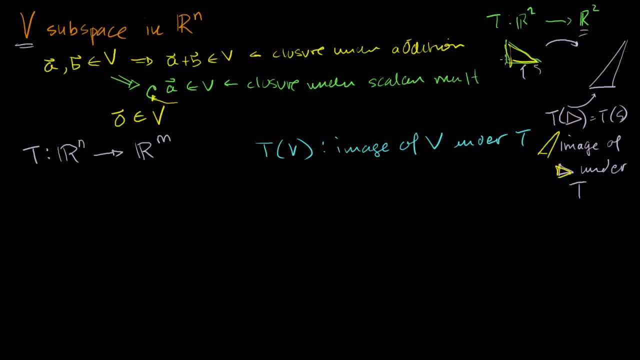 you and just as a bit of a reminder, in that last video, these triangles didn't, These weren't subspaces, And just as you could take scalar multiples of some of the vectors that are subsets, that are members of this triangle, 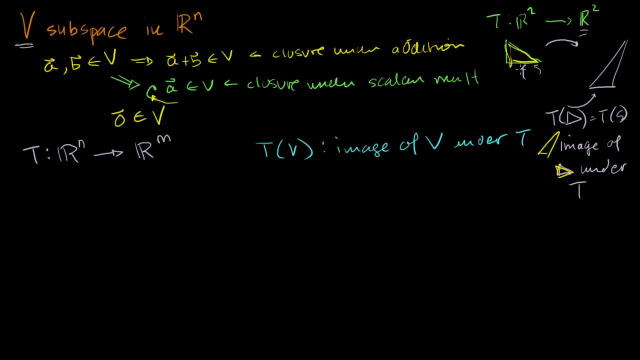 and you'll find that they're not going to be in that triangle. So this wasn't a subspace. This was just a subset of R2.. All subsets are not subspaces, but all subspaces are definitely subsets, Although something can be a subset of itself. 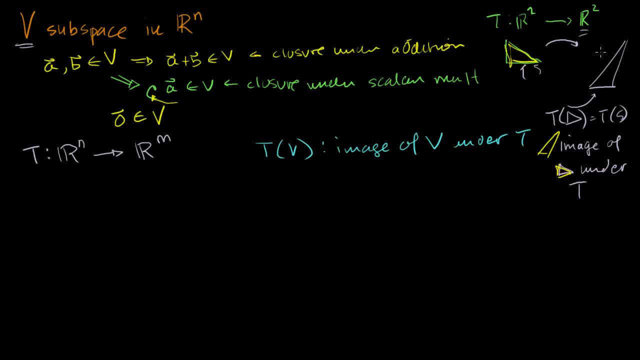 I don't want to wander off too much, But this just helps you visualize what we mean by an image. It means all of this, All of the vectors that are mapped to from the members of your subset. So I want to know whether the image of V under T is a. 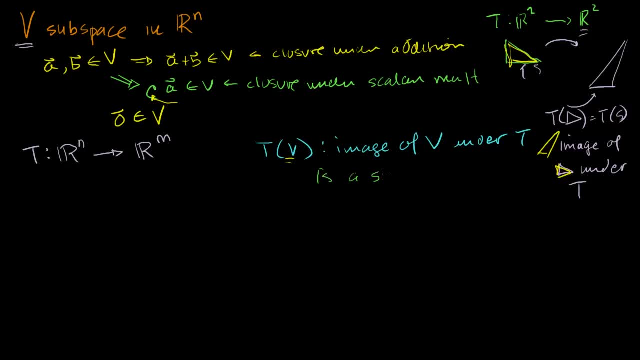 subspace. So, in order for it to be a subspace, if I take the transformation, let me find two members of T. Well, clearly, if I take the transformation of any member members of v, I'm getting members of the image. 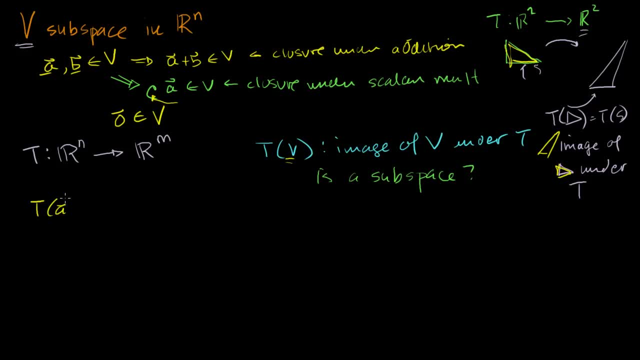 So I can write this Clearly: the transformation of a and the transformations of b, these are both members of our images of v under t. These are both members of that right there. So my question to you is: what is the transformation of a? 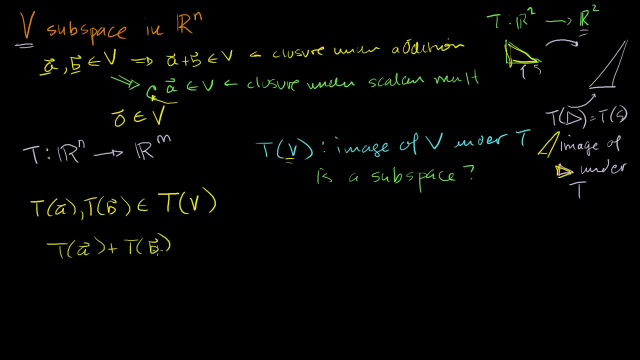 plus the transformation of b And the way I've written this. these are two arbitrary members of our image of v under t, or maybe I should call it t- of capital V. These are two arbitrary members, So what is this equal to? 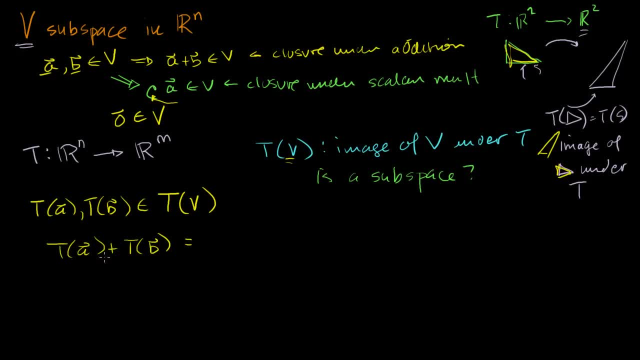 Well, we know from our properties our definition of linear transformations. this is equal to the sum of the transformations of two vectors- is equal to the transformation of the sum of their vectors. Now is the transformation of a plus b. is this a member? 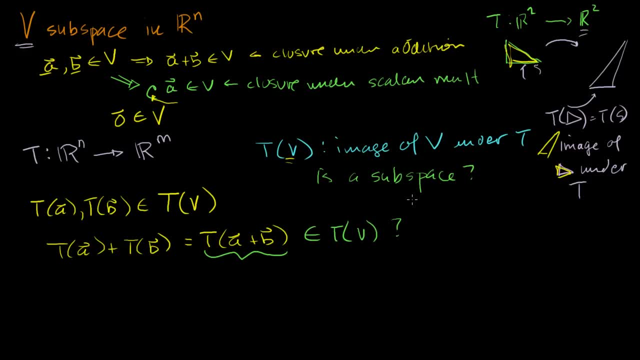 of t v. Is it a member of our image? Well, a plus b is a member of v and the image contains the transformation of all of the members of v. So the image contains the transformation of this guy. This guy, a plus b, is a member of v. 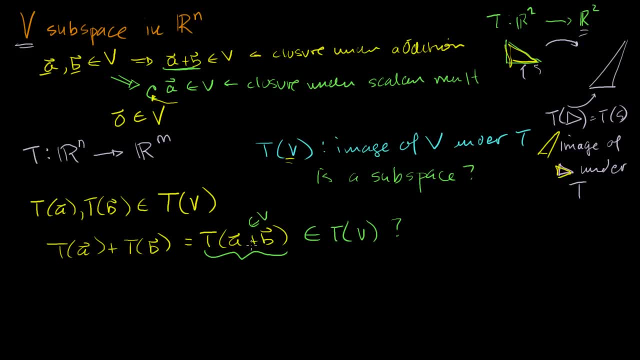 So you're taking the transformation of a member of v which, by definition, is in your image of v under t. So this is definitely true. Now let's ask the next question. If I take a scalar multiple of some member of my image of v, 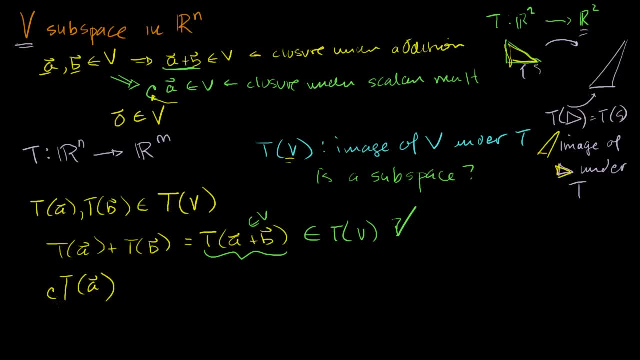 under t, or my t of capital V, right there. what is this equal to? by definition, for a linear transformation, This is the same thing as a transformation of the scalar times, the vector. Now, is this going to be a member of our image of v under t? 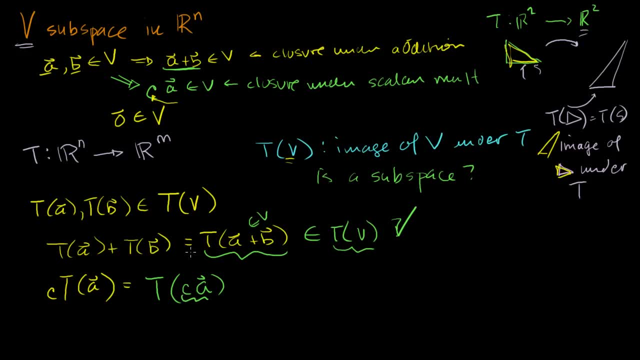 Well, we know that ca is definitely in v. right, That's from the definition of a subspace. This is definitely in v, And so if this is in v, the transformation of this has to be in v's image under t. 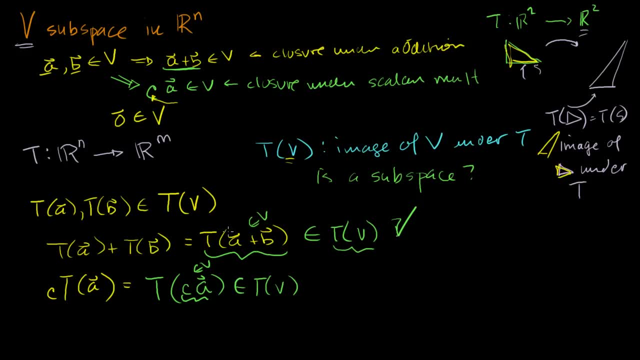 So this is also a member of v And obviously you can set this equal to 0.. The 0 vector is a member of v, So any transformation of if you just put a 0 here, you'll get the 0 vector. 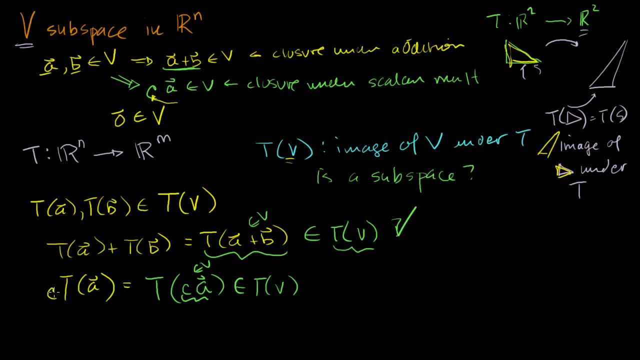 So the 0 vector is definitely. I don't care what this is. if you multiply it times 0, you're going to get the 0 vector. So the 0 vector is definitely also a member of Tv. So we come on the result that the image of v under t is a. 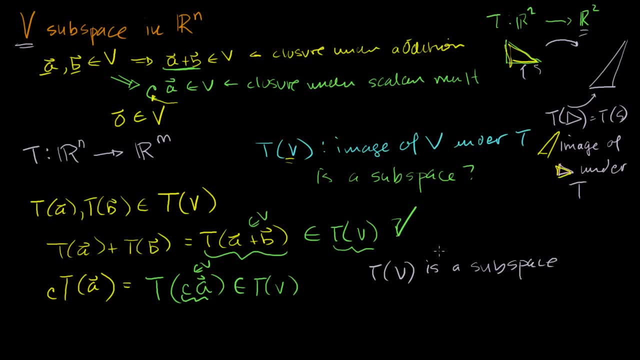 subspace, which is a useful result which we'll be able to use later on. But this, I guess, might naturally lead to the question: what if we? What if we go? you know, everything we've been dealing with so far have been subsets in the case of this triangle. 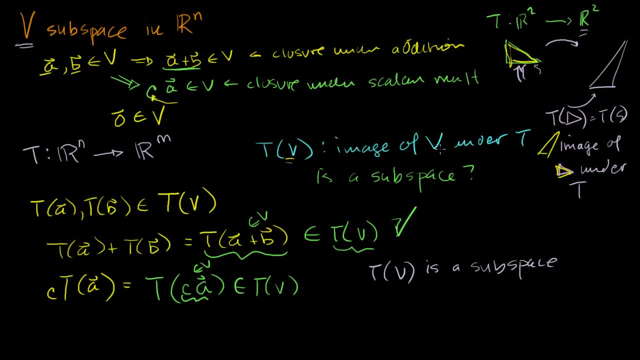 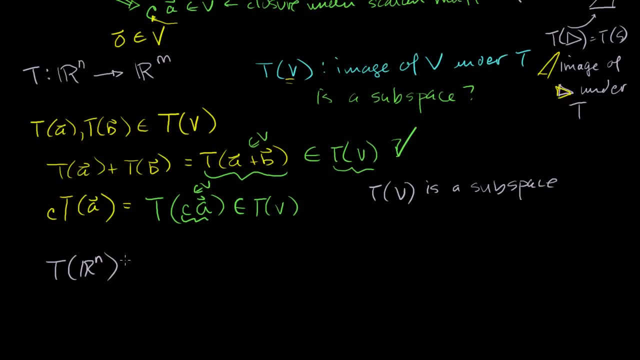 or subspaces in the case of v. But what if I were to take the image of Rn under t? right, This is the image of Rn under t. Let's think about what this means. This means: what do we get when we take any member of? 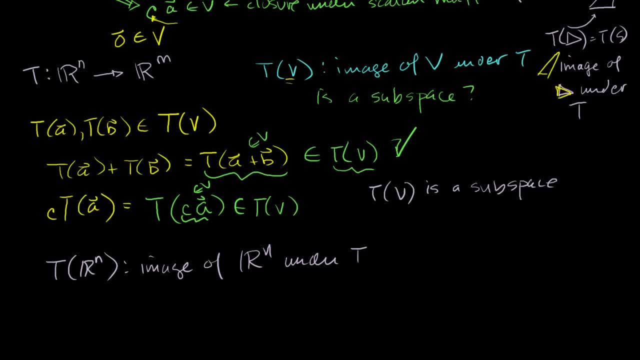 Rn. what is the set of all of the vectors? that when we take the transformation of all of the members of Rn, Let me write this: This is equal to the set of the transformation of all of the x's, where each x is a member of Rn. 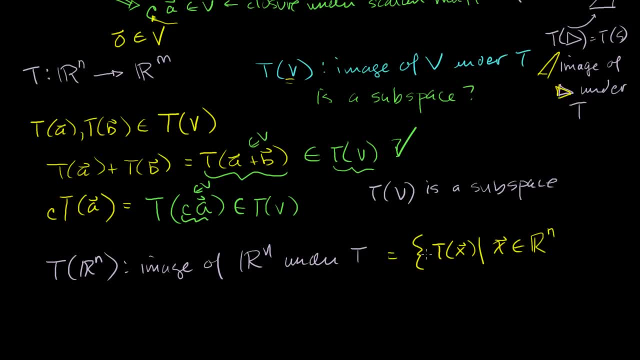 So you take each of the members of Rn and transform them and you create this new set. This is the image of Rn under t, The image of Rn under t. Well, there's a couple of ways you can think of this. 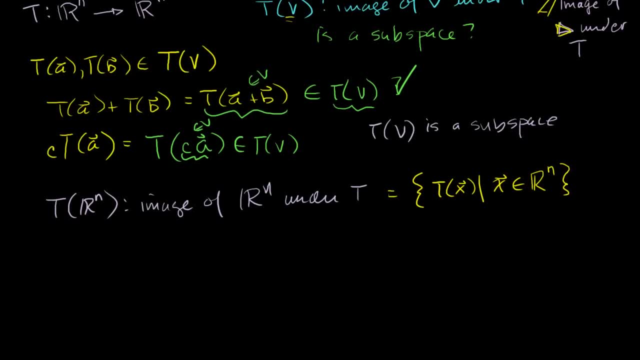 This is remember- when we defined- let's see, t is a mapping from Rn to Rm- We defined this as the domain, all of the possible inputs for our transformation, and we defined this the codomain. And remember I told you that the codomain is essentially 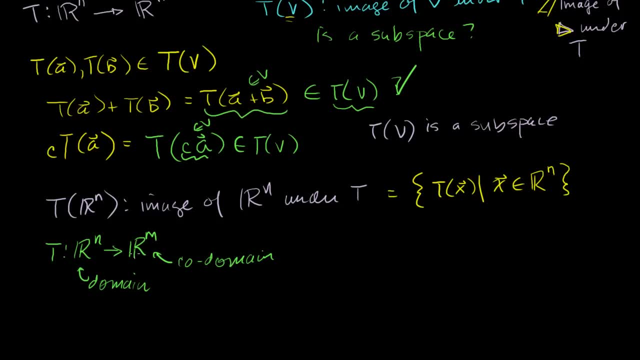 it's part of the definition of the function or of the transformation and it's the space that we map to. It's not necessarily all of the things that we're mapping to, For example, the image of Rn under transformation, maybe. 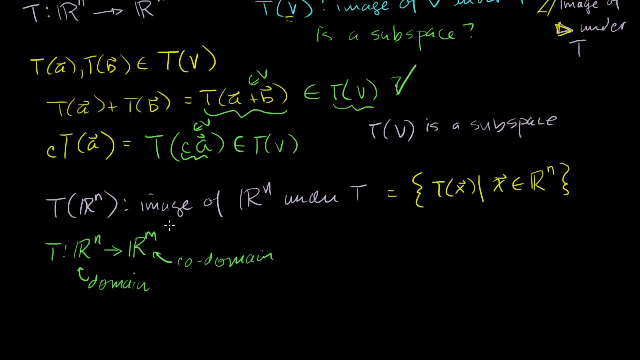 it's all of Rm or maybe it's some subset of Rn. The way you can think about it- and I touched on this in that first video- is: and they'll never- or at least the linear algebra books I looked at- they didn't specify this. 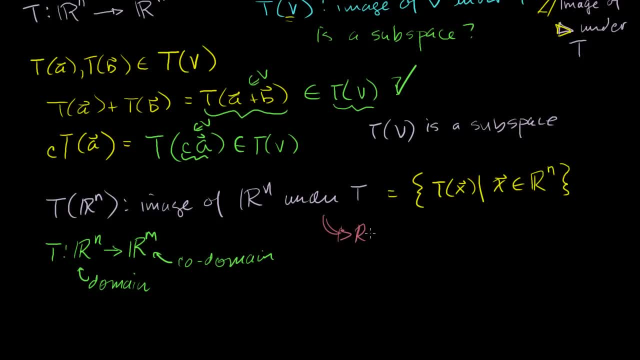 But you can kind of view this as the range of t. These are the actual members of Rm that t maps to That. if you take the image of Rn under t, you're actually finding. so let me say this is, let's say that Rm looks like. 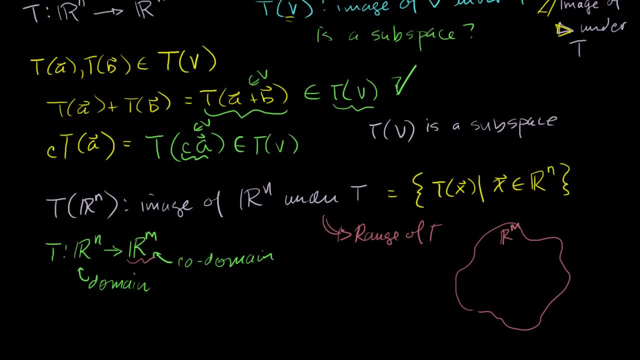 that Rm. obviously it'll go in every direction. And let's say that when you take let me draw Rn right here, say this is Rn And we know that t is a mapping from Rn to Rm. 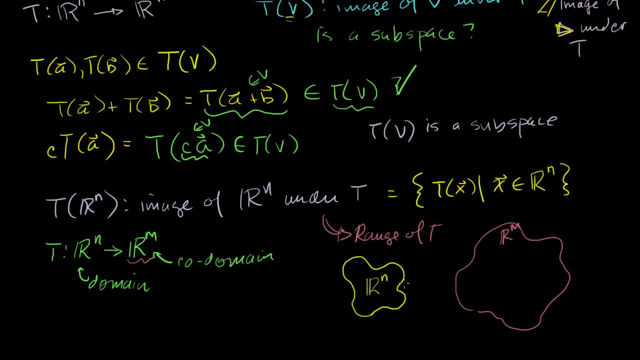 But let's say, when you take every element of Rn and you map them into Rm, Let's say you get Rn. Let's say you get Rn. Let's say you get Rn. Let's say you get some subset of Rm. 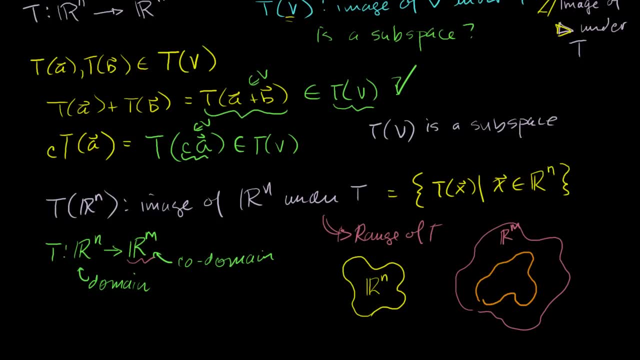 Let's say you get something that looks like this. So let me see if I can draw this nicely, So you literally map every point here and it goes to one of these guys, Or one of these guys can be represented as a mapping from: 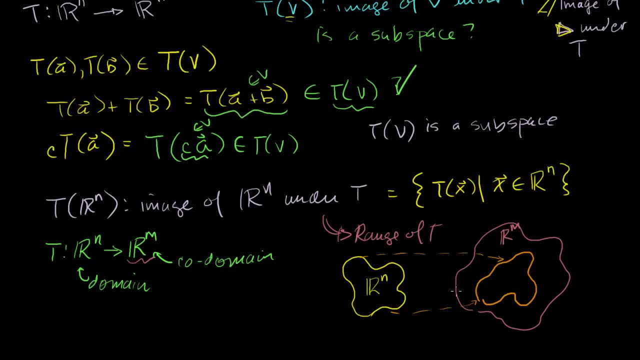 one of these members right here. So if you map all of them you get this subset right here. This subset is: this: is t, the image of Rm, The image of Rn under t And in the terminology that you don't normally see in linear. 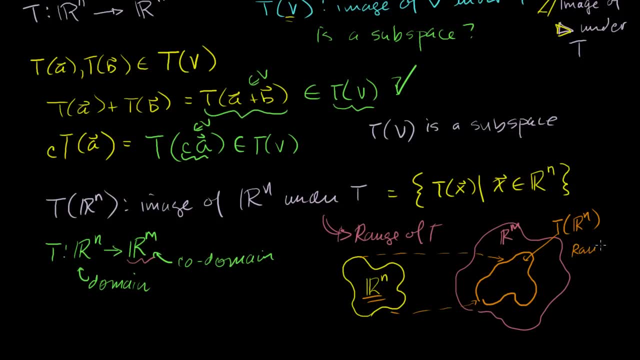 algebra a lot. you can also kind of consider it its range, The range of t. Now, this has a special name. This is called, and I don't want you to get confused- this is called the image of t, Image of t. 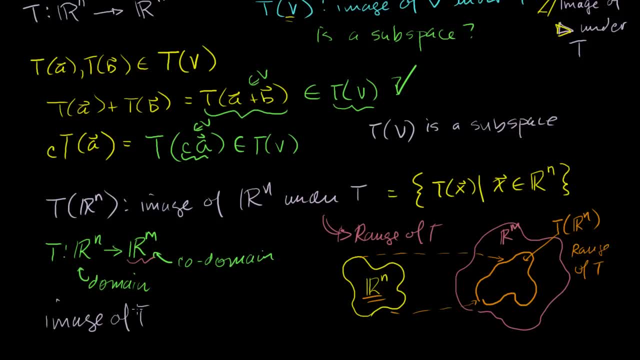 And it might be a little confusing- Image of t. So this is- it's sometimes written as Just Im of t. Now, you're a little confused here. You're like you know, before, when we were talking about subsets, we would call this the image of our subset under t. 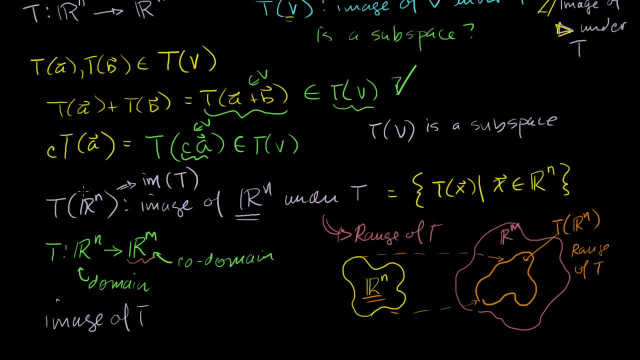 And that is the correct terminology when you're dealing with a subset. But when you take all of a sudden the entire n-dimensional space and you're finding that image, we call that the image of the actual transformation. So we can also call this set right here. we can call this: 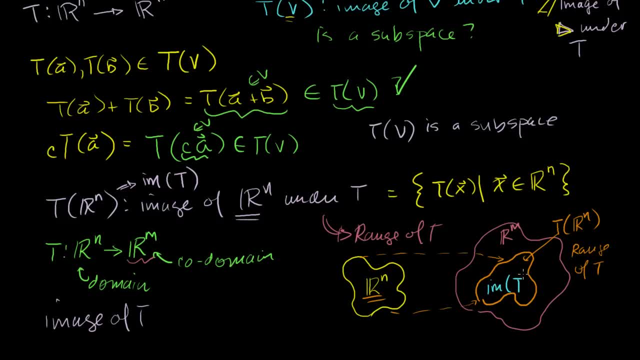 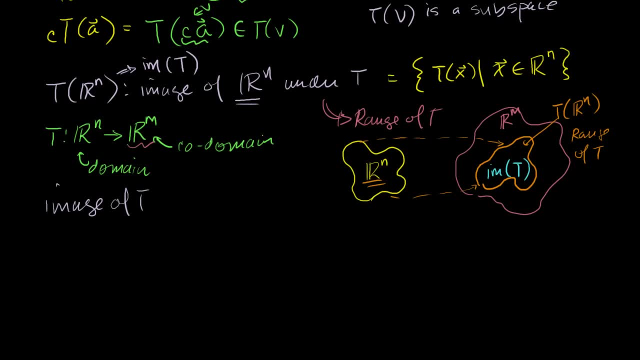 the image, The image of t. And now, what is the image of t? Well, we know that we can write any, And this is, you know, literally any. So t is going from rn to rm. We can write t, t of x. 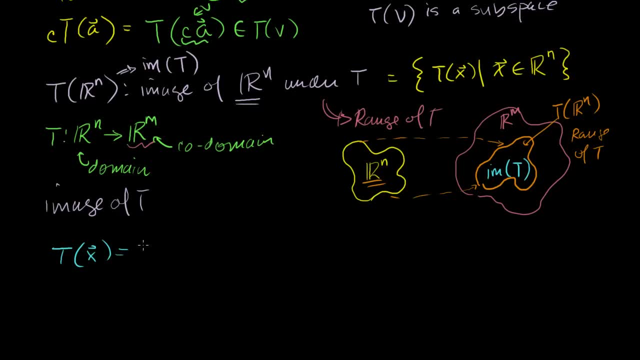 We can write any linear transformation like this as being equal to some matrix, some m by n matrix m by n times a vector, And these vectors obviously are going to be members of Rn times, some Rn, And what is this? 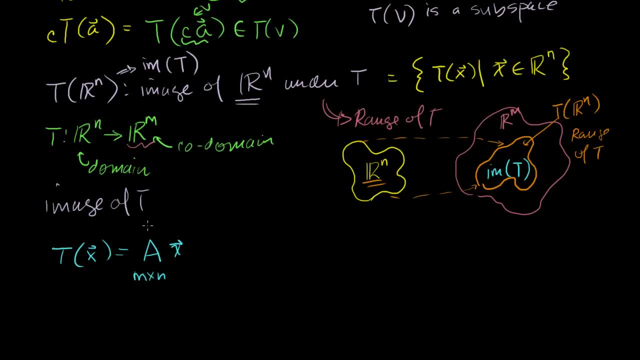 So what is the image? Let me write it in a bunch of different ways. What is the image of Rn under T? So we could write that as T of Rn, which is the same thing as the image of T. Notice, we're not saying under anything else, because now 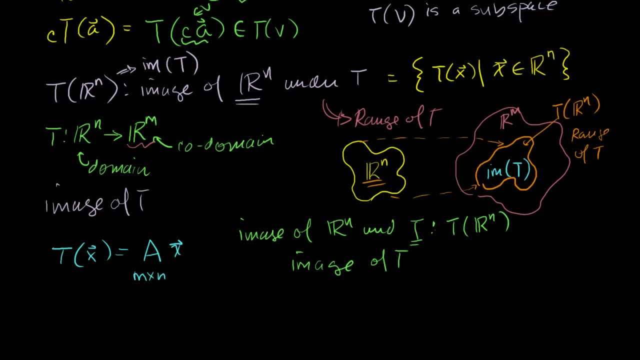 we're saying the image of the actual transformation, which we could also write as the image of T. Well, what are these equal to? These are equal to the sets of all the transformations of x. Well, all the transformations of x are going to be Ax. where? 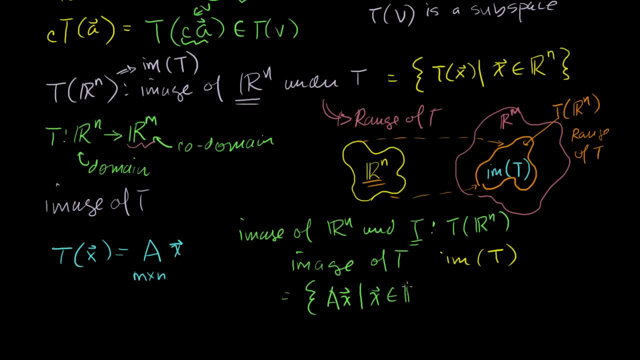 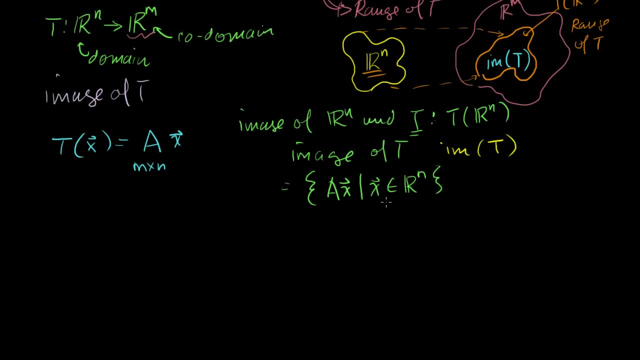 So x is going to be an n-tuple where each element just has to be a real number. So what is this? So if we write A, let me write my matrix A. It's just a bunch of column vectors: A1, A2.. 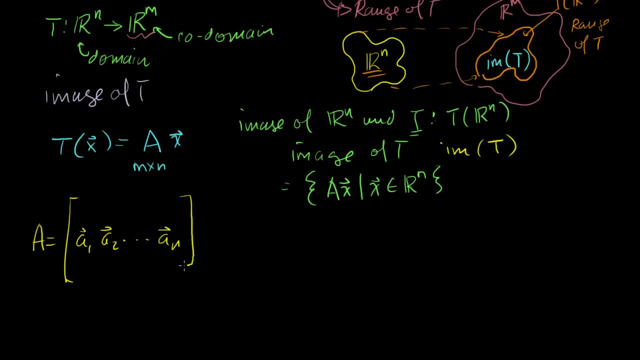 It's going to have n of these because it has n columns And so A times Rn. So if I multiply that times any x that's a member of Rn. so I multiply x1,, x2, all the way to xn. we've seen this multiple. 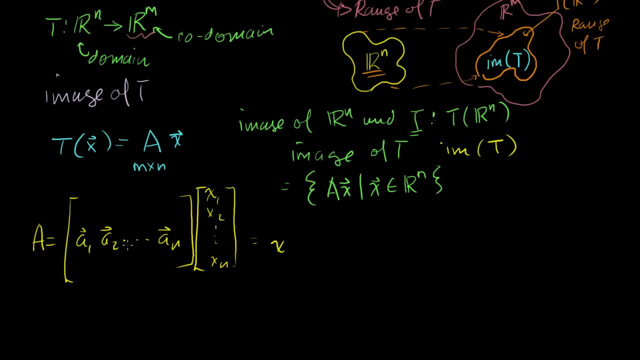 multiple times. This is equal to x1, the scalar x1, times A1, plus x2 times A2, all the way to plus xn times An. And we're saying we want the set of all of these sums, of these column vectors.